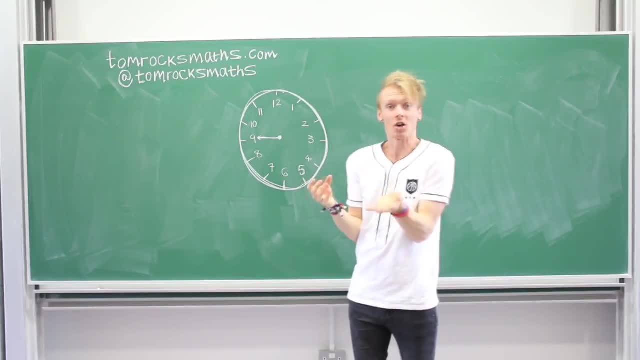 a circle, but this is our 12 hour clock and it's currently nine o'clock, so our hand is pointing to nine. Now, if we let six hours of time pass, what will the time be? If you look at the clock, it's. it's not too tricky, you know. you can probably all do it in your head: nine o'clock, six hours. 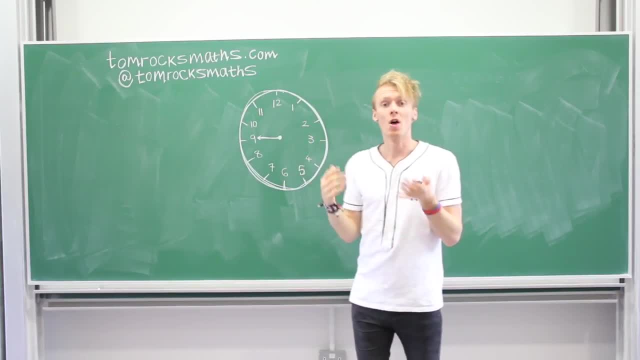 of time Passes- one, two, three, four, five, six, it goes to three o'clock. but nine plus six does not equal three, and that's the trick here. that's where the sort of underlying modular arithmetic that's hidden in the 12 hour clock sort of comes out of the woodwork, because what we're doing with a clock is 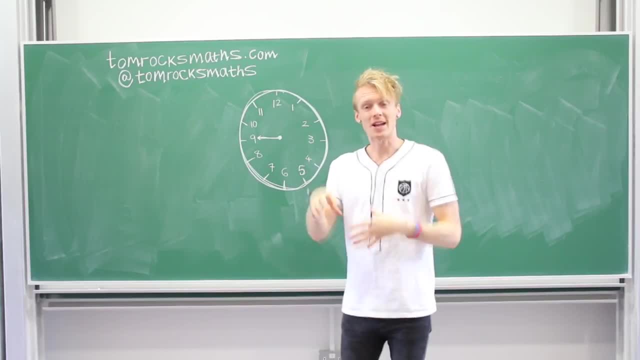 doing arithmetic modular 12. so that simply means that when you get to 12 you then start again. the numbers start to change. So it's sort of wrap around. and it looks a bit easier when you draw it out as a circle of numbers like this, like a clock, because you just sort of go nine, ten, eleven, twelve and then you start again. 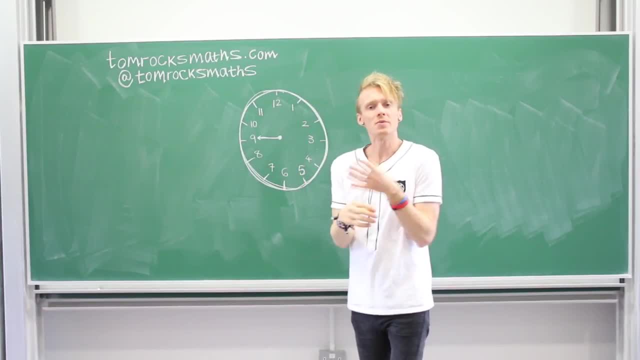 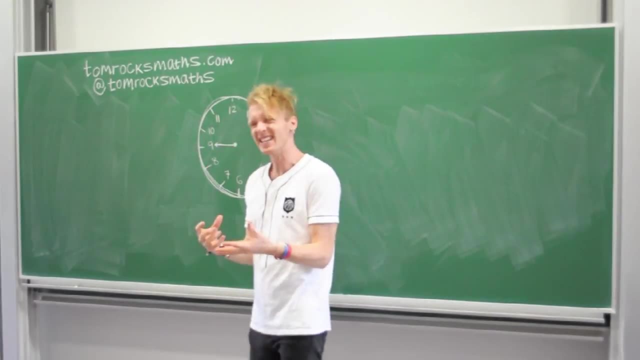 one, two, three and you keep going round. so if it was nine o'clock and then 12 hours pass, the hand will go all the way around the circle back to nine. so it's still nine o'clock, but nine plus 12 again, it doesn't equal nine in normal time. 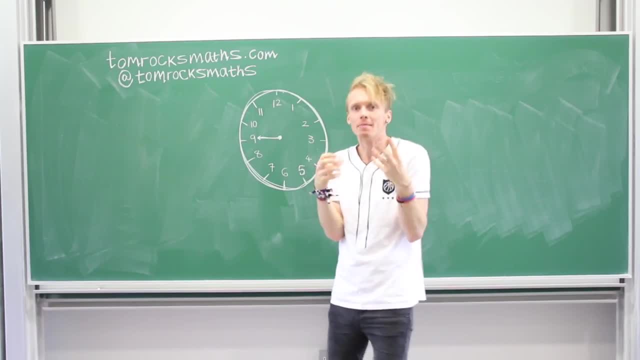 In normal arithmetic- and that's sort of what's going on with modular arithmetic- you have a set number and once you get to that number- in this case 12- you just start again. you just ignore the fact that 12 has already passed. you're only interested in the bit beyond 12 or beyond. 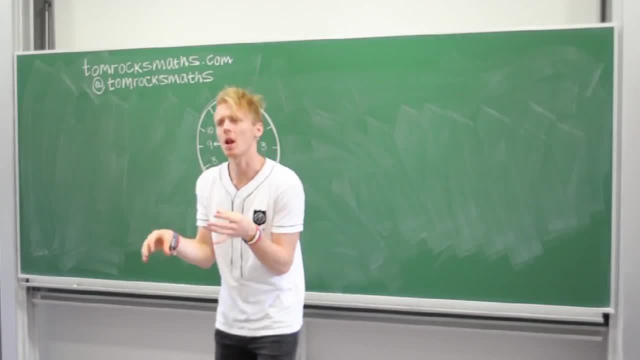 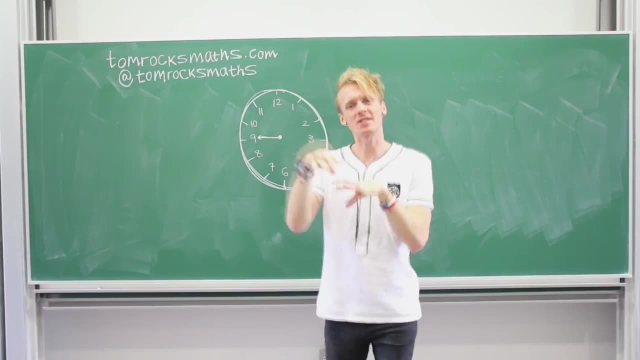 multiples of 12.. So let's think about the clock mathematically, so sort of, from the modular arithmetic point of view. so nine o'clock plus six hours, we all know, is three o'clock, but nine plus six gives you 15.. So why is 15 equal to three o'clock? 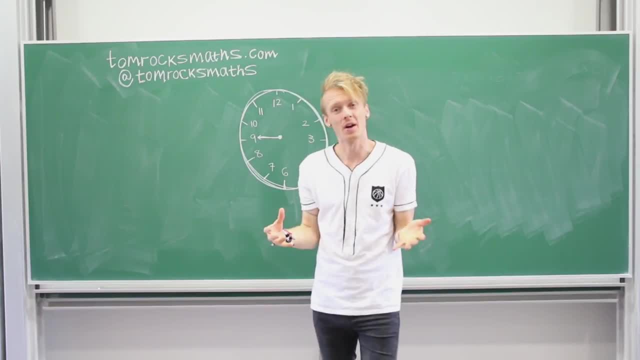 Well, it's to do with the fact that the clock is modular 12, because you start at nine, you then add your six, you get 15. but, importantly, 15 contains one group of 12, and so it doesn't matter that. that's there. we sort of ignore that in some sense. it's not. 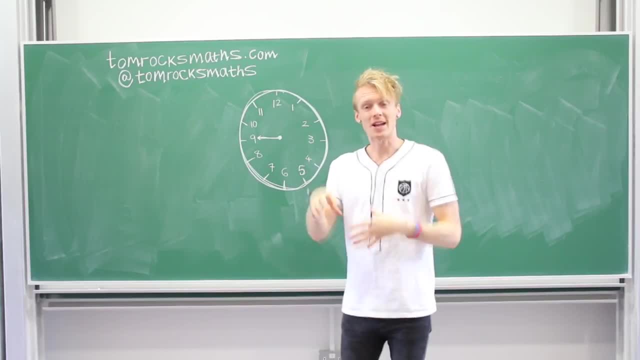 doing arithmetic modular 12.. So that simply means that when you get to 12 you then start again. the numbers start to change. So it's sort of wrap around. and it looks a bit easier when you draw it out as a circle of numbers like this, like a clock, because you just sort of go nine, ten, eleven, twelve and then you start again. 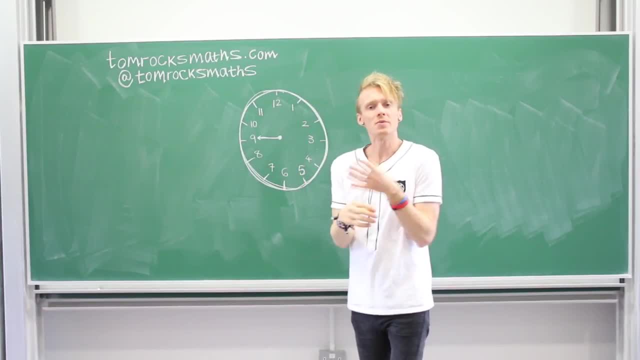 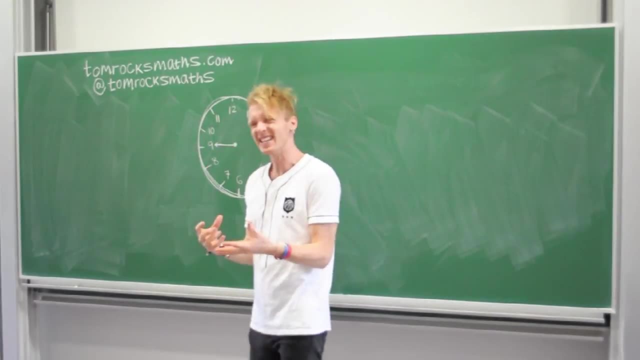 one, two, three and you keep going round. so if it was nine o'clock and then 12 hours pass, the hand will go all the way around the circle back to nine. so it's still nine o'clock, but nine plus 12 again, it doesn't equal nine in normal time. 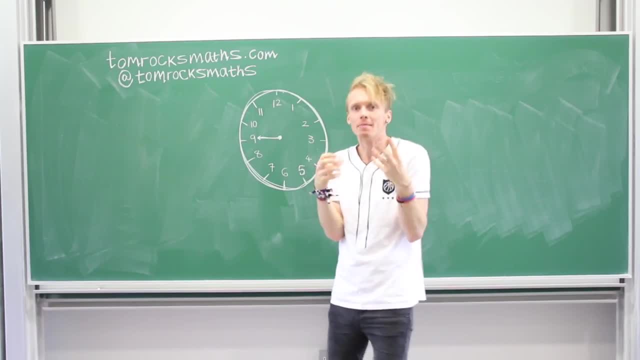 In normal arithmetic- and that's sort of what's going on with modular arithmetic- you have a set number and once you get to that number- in this case 12- you just start again. you just ignore the fact that 12 has already passed. you're only interested in the bit beyond 12 or beyond. 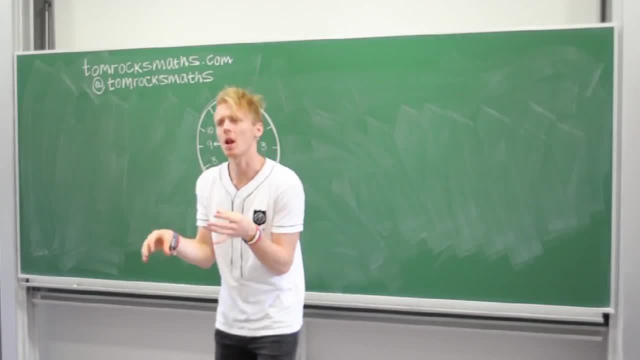 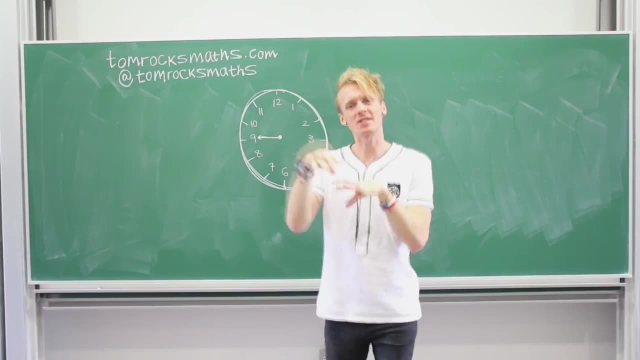 multiples of 12.. So let's think about the clock mathematically, so sort of, from the modular arithmetic point of view. So nine o'clock plus six hours, we all know, is three o'clock, but nine plus six gives you 15.. So why is 15 equal to three o'clock? 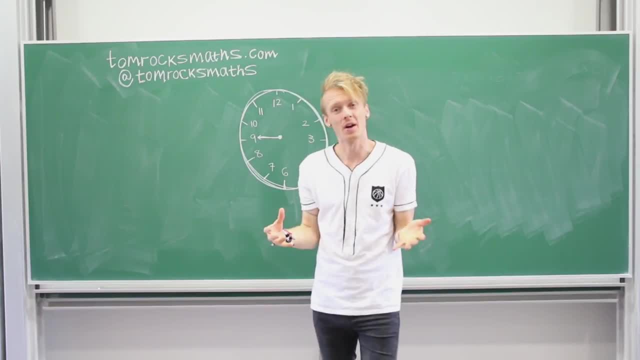 Well, it's to do with the fact that the clock is modular 12, because you start at nine, you then add your six, you get 15. but, importantly, 15 contains one group of 12, and so it doesn't matter that. that's there. we sort of ignore that in some sense. it's not. 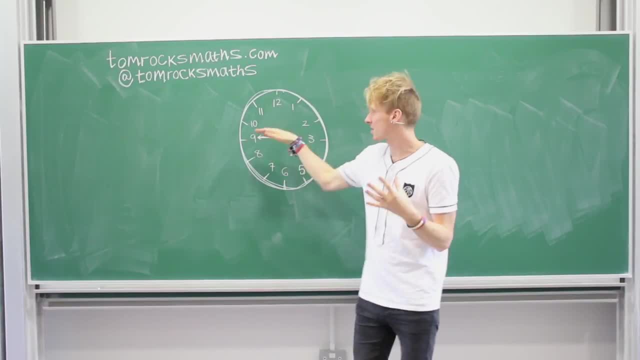 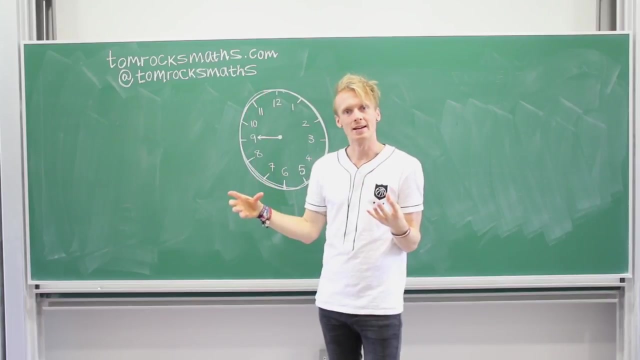 relevant. so that first group of 12, which is like us, counting up the first three hours to 12. we just ignore that and we only care about the remainder, so the bit beyond 12.. So in the case of nine plus six, you sort of go to 12, and then there's another three from 12 to 15, and that's why nine o'clock. 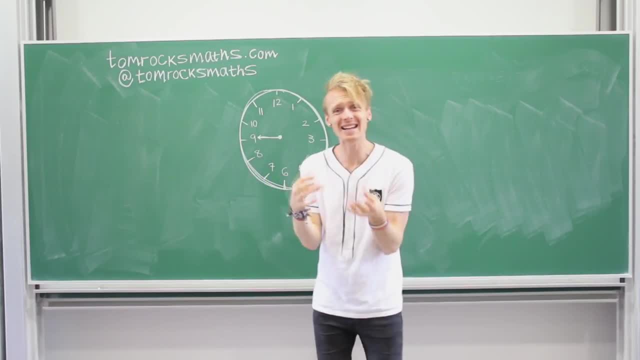 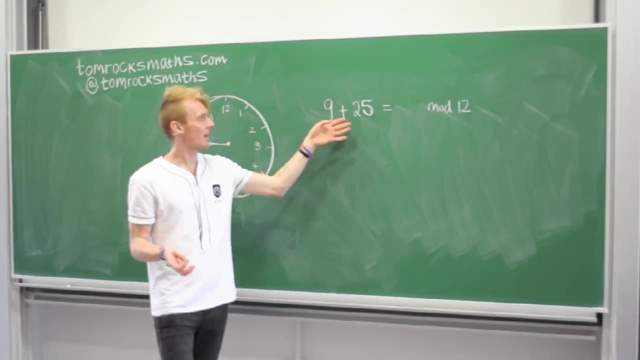 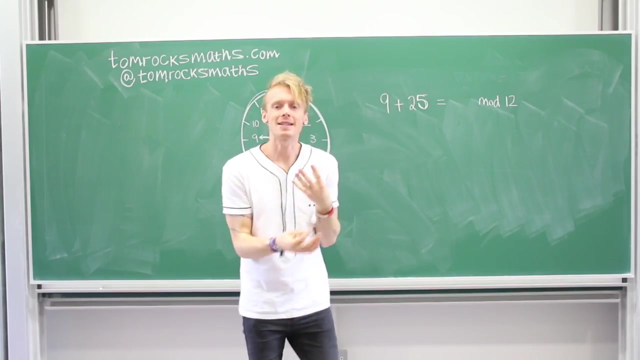 plus six hours goes to three o'clock, and it works exactly the same with any other number and with any other form of modular arithmetic. So say we want to work out nine plus 25, mod 12. All we're going to do here is add nine and 25 and 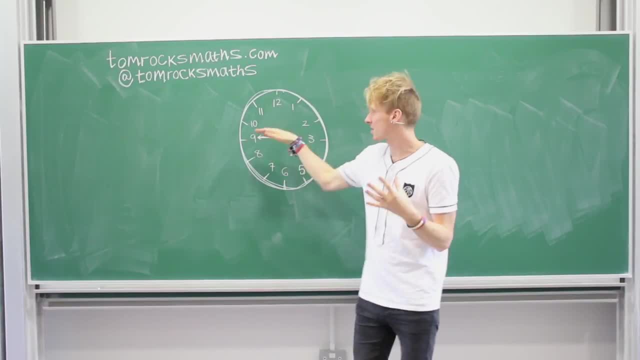 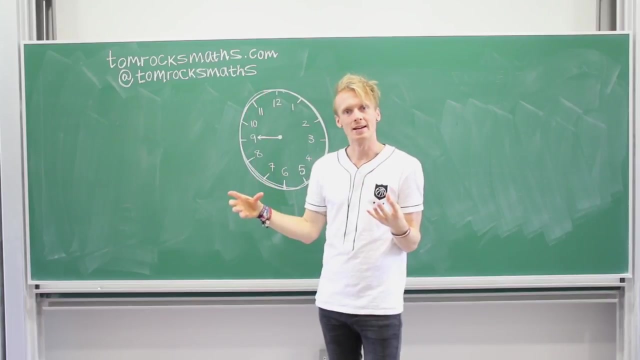 relevant. so that first group of 12, which is like us, counting up the first three hours to 12. we just ignore that and we only care about the remainder, so the bit beyond 12.. So in the case of nine plus six, you sort of go to 12, and then there's another three from 12 to 15, and that's why nine o'clock. 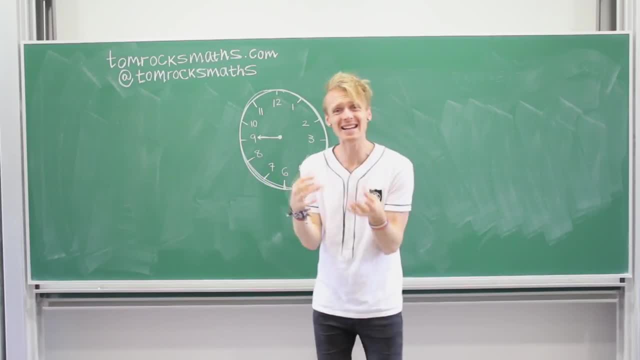 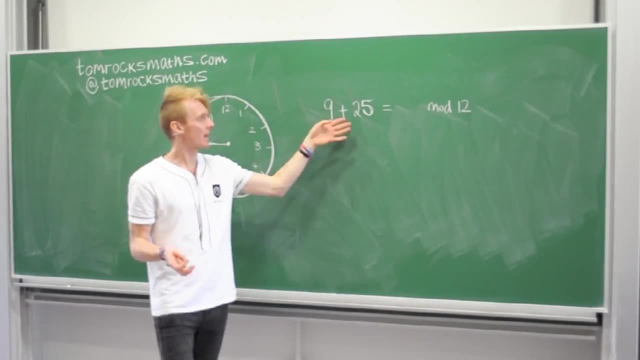 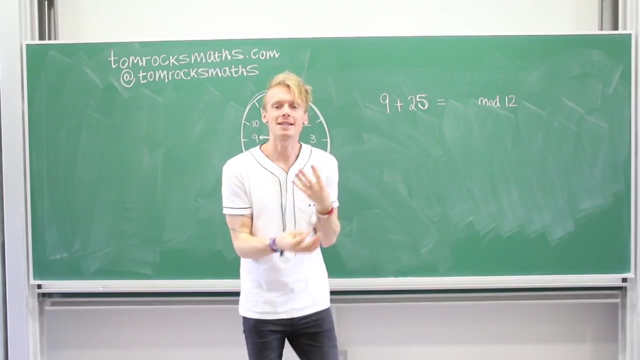 plus six hours goes to three o'clock, and it works exactly the same with any other number and with any other form of modular arithmetic. So say we want to work out nine plus 25 mod 12. All we're going to do here is add nine and 25. 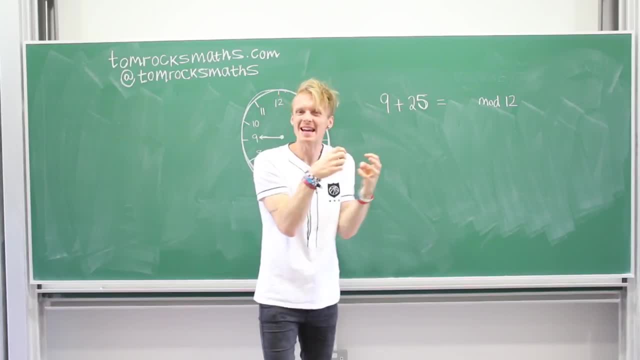 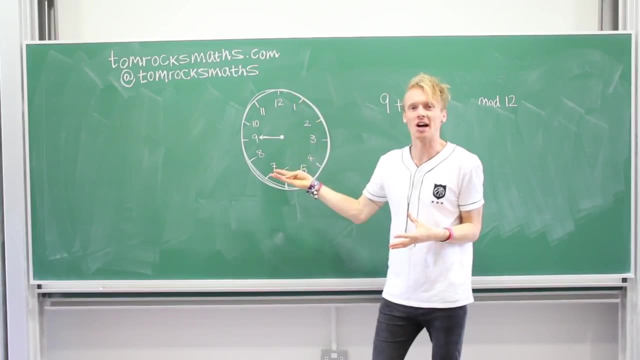 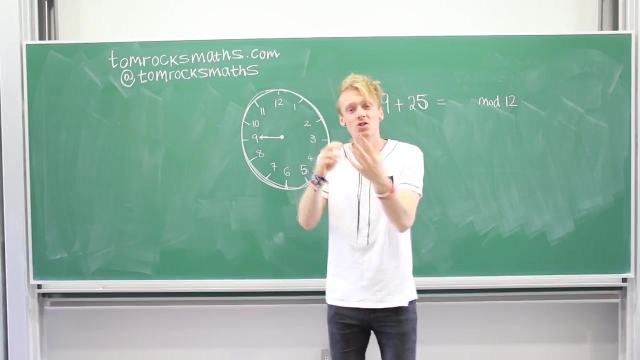 and then think about what's the remainder left once you take out your groups of 12.. So you can also think of it in terms of time. so again, if it's nine o'clock and then 25 hours pass, we sort of know that there are 24 hours in a day, but that's just two. lots of. 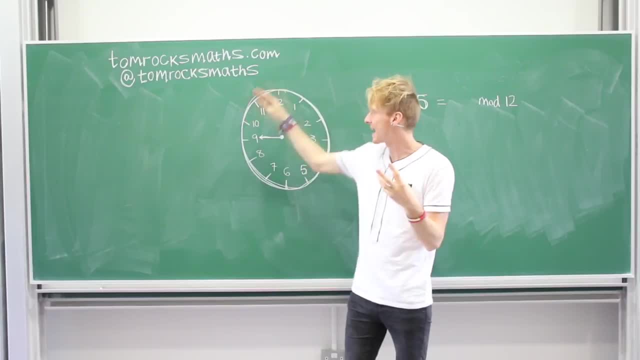 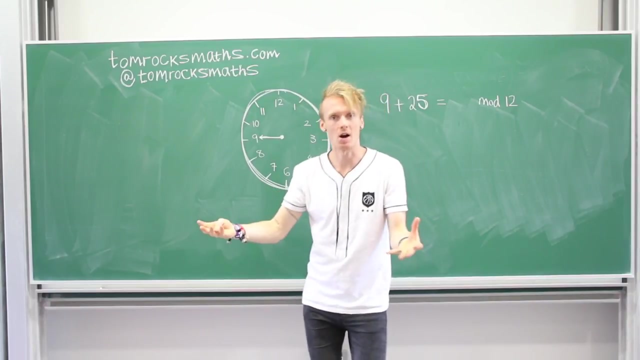 12.. So it's two whole sort of rotations of the clock by the hour hand and you do the two whole rotations for your first 24 that you're adding on and then you've just got one more. so nine plus 25, in terms of time, would just take you to 10 o'clock, and it's the same with the maths, because nine plus 25 it's. 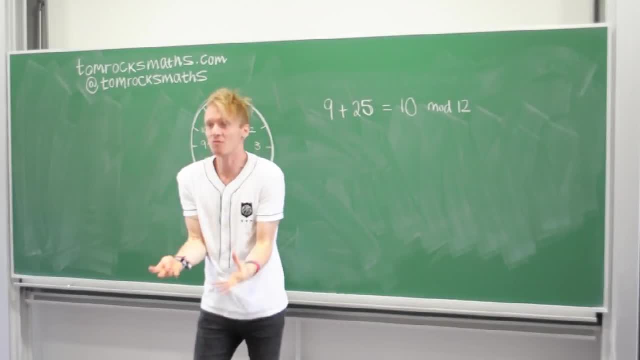 just 10 mod 12.. For exactly that reason that we just sort of went through with the clock, the first two groups of clock are not the same. So that's the whole rotation of the clock, and that's the whole rotation of the clock. 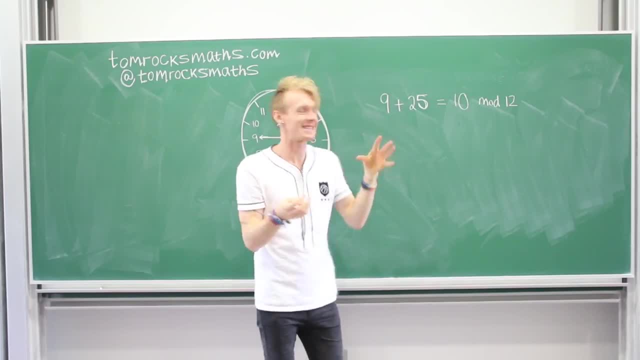 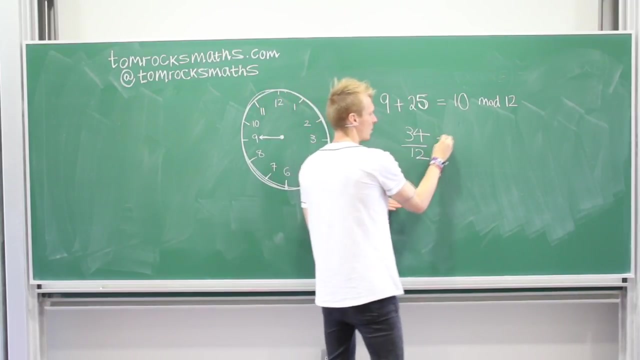 12, they don't matter. so what you're sort of doing is adding 9 and 25 in the normal way to get, say, 34, and then you're thinking to yourself: okay, how many 12s go into 34? so, 34 divided by 12, well, there's 2, and then there's remainder 10. 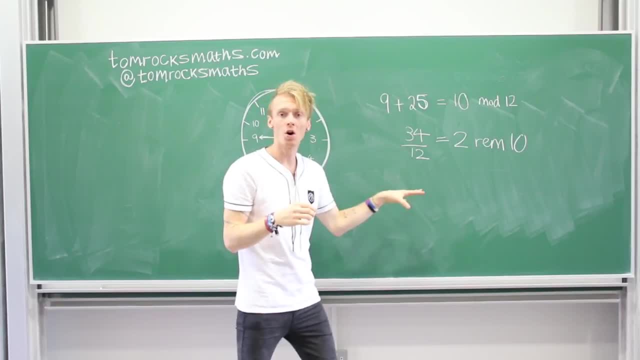 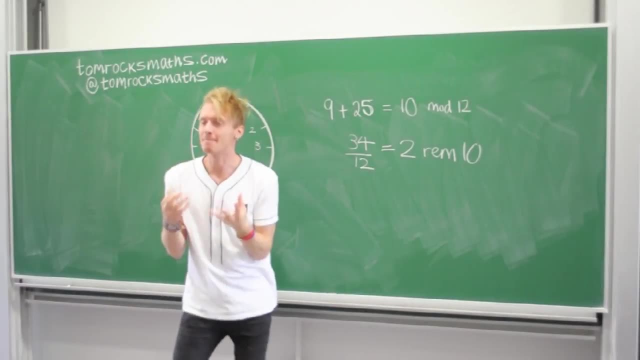 because 2 lots of 12 give you the 24, and then there's another 10, so it's 2 and remainder 10. but this 2 it doesn't matter in modular arithmetic because you've got 2 lots of 12 and we don't really care about them. we like ignore. 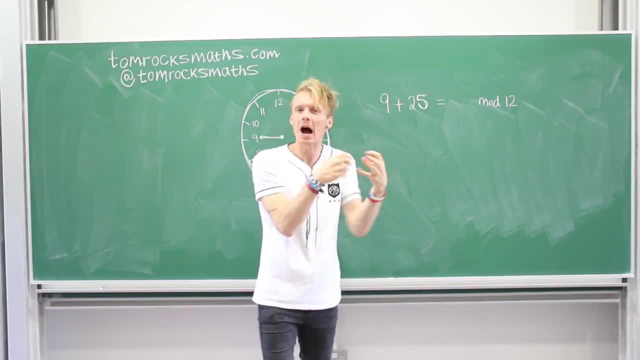 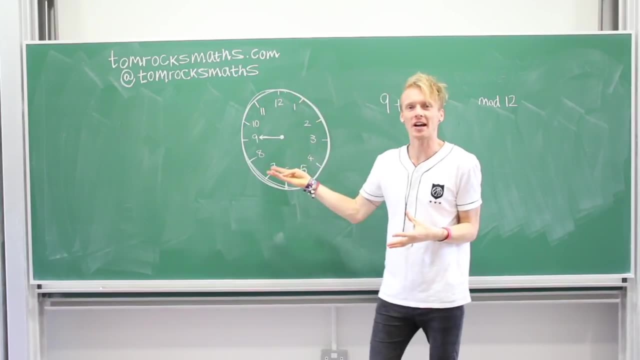 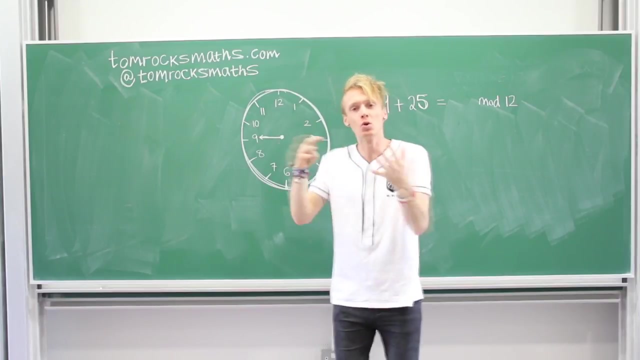 then think about what's the remainder left once you take out your groups of 12.. So you can also think of it in terms of time. so again, if it's nine o'clock and then 25 hours pass, we sort of know that there are 24 hours in a day, but that's just two lots of 12.. 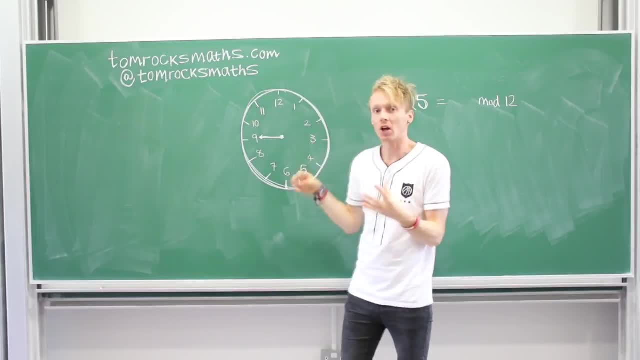 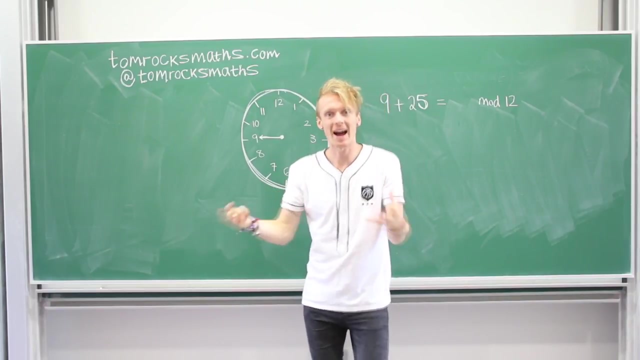 So it's two whole sort of rotations of the clock by the hour hand and you do the two whole rotations for your first 24 that you're adding on and then you've just got one more. so nine plus 25, in terms of time, would just take you to 10 o'clock, and it's the same with the maths, because nine plus 25 it's. 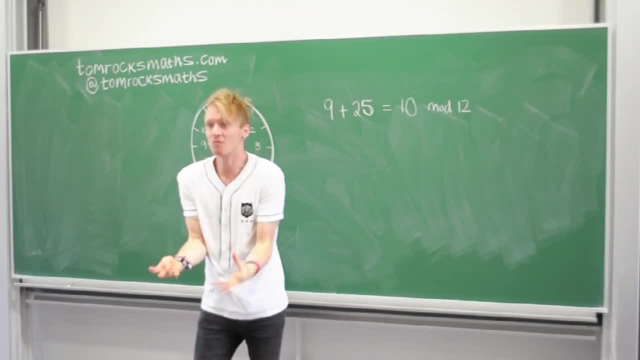 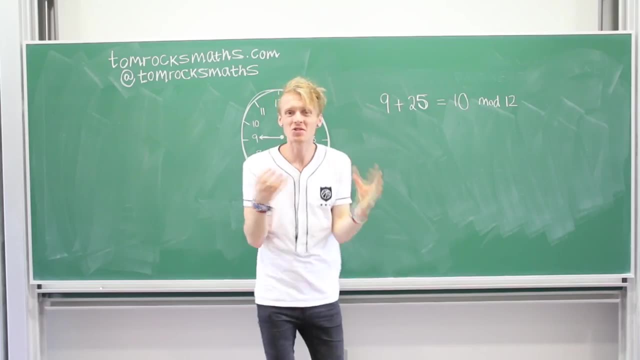 just 10 mod 12.. For exactly that reason that we just sort of went through with the clock, the first 12 they don't matter. so what you're sort of doing is adding 9 and 25 in the normal way to get, say, 34. 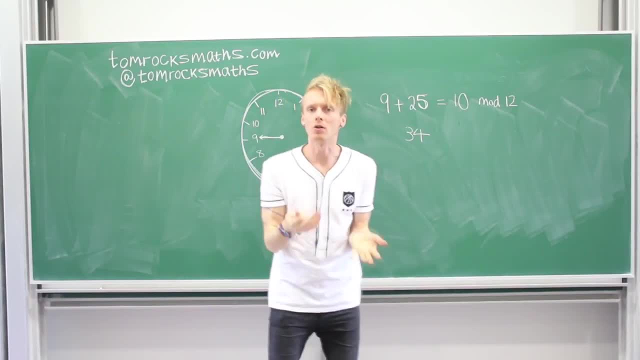 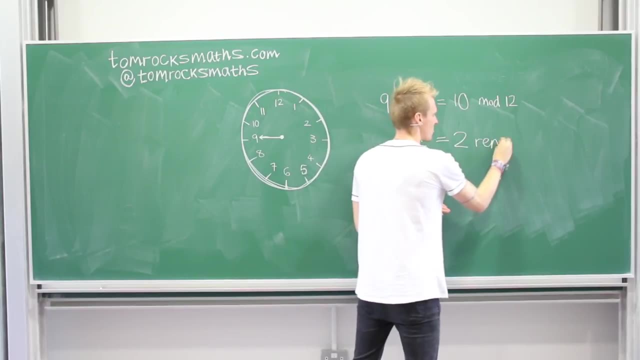 and then you're thinking to yourself: okay, how many 12s go into 34.. So 34 divided by 12, well, there's 2, and then there's remainder 10, because two, lots of 12 give you the 24, and then there's another 10. 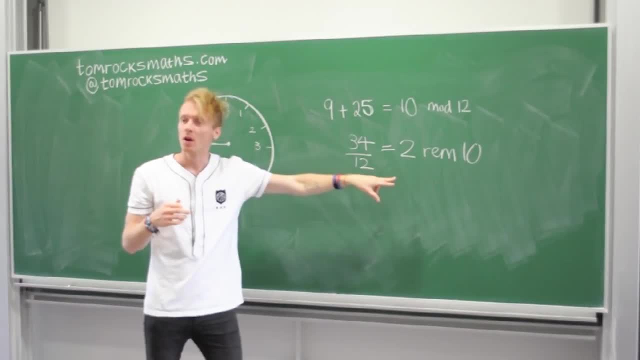 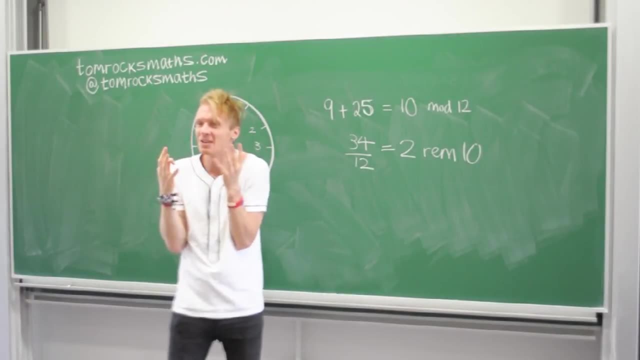 so it's 2 and remainder 10.. But this 2 it doesn't matter in modular arithmetic, because you've got two lots of 12 and we don't really care about them, we like ignore them. and so here this two lots of 12, it doesn't matter, it's just. 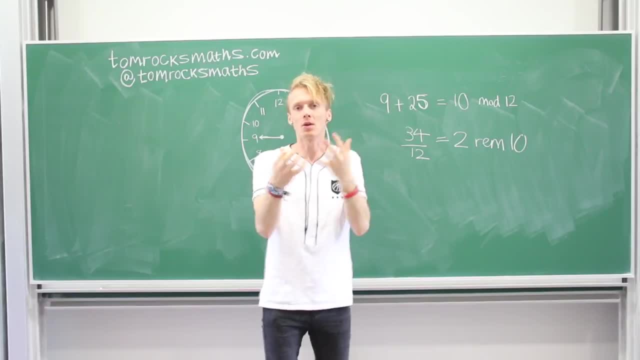 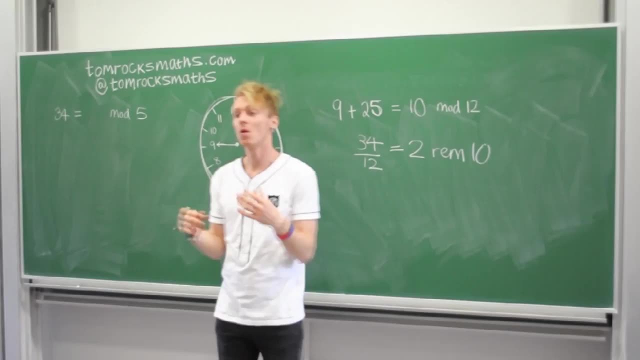 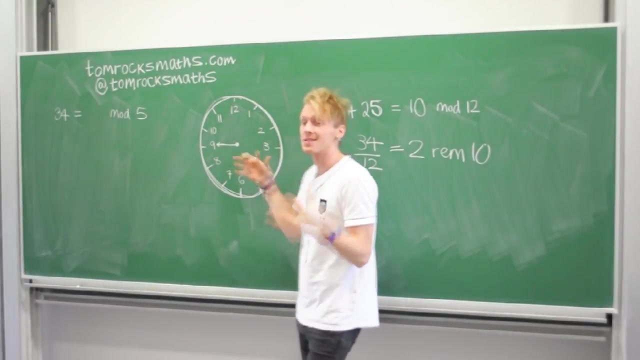 the remainder being 10. that's the key in terms of modular arithmetic. that's the only bit that we care about, and so that's why the answer is just 10 mod 12.. All of the examples I've done so far, of course, have been mod 12, and that's because we were thinking about things in terms of the 12th. 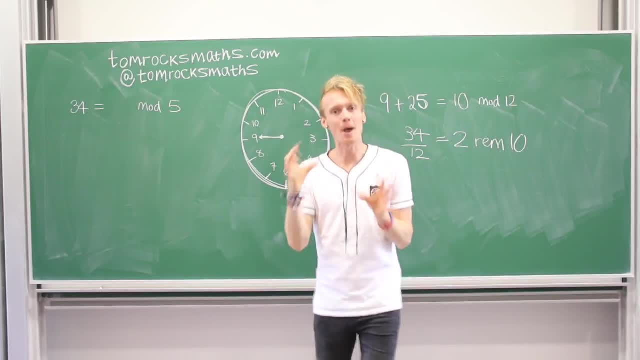 So mod 12 is the number of our clock, which is mod 12, but of course you can use any number. so let's take 34, which is our 9 plus 25.. Let's think about what 34 is in say mod 5.. Okay, so we proceed in the 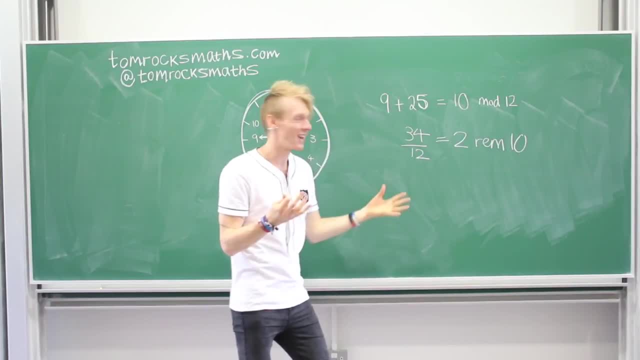 them, and so here this 2, lots of 12, it doesn't matter, it's just the remainder being 10. that's the key in terms of modular arithmetic. that's the only bit that we care about, and so that's why the answer is just 10 mod 12. all of the 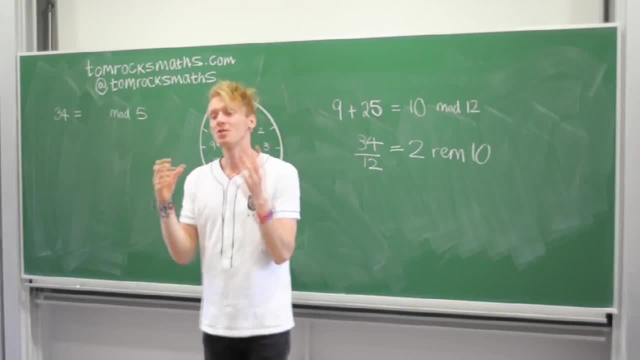 examples I have done so far, of course, have been mod 12, and that's because we've got a lot of 12s and we've got a lot of 12s and we've got a lot of 12s. we were thinking about things in terms of the 12 hour clock, which is mod 12, but 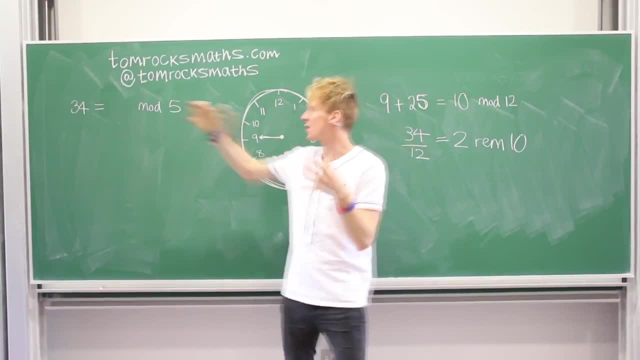 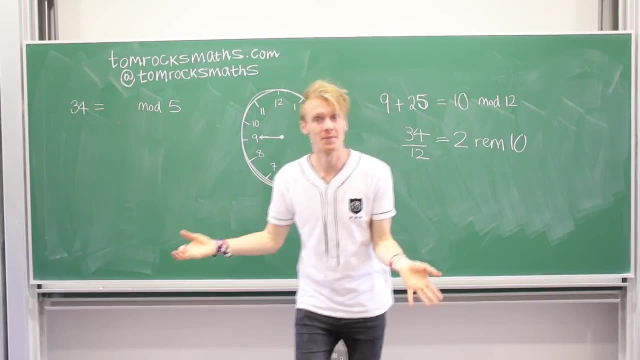 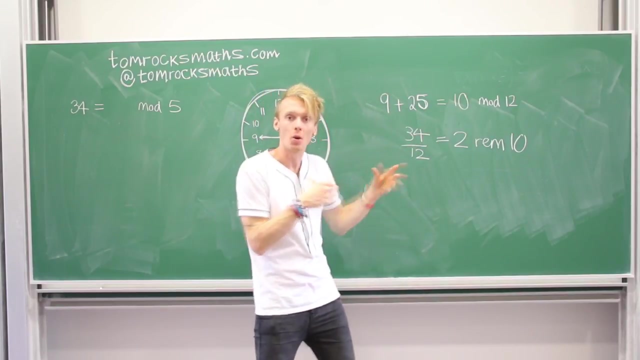 of course you can use any number. so let's take 34, which is our 9 plus 25. let's think about what 34 is in, say, mod 5. okay, so we proceed in the same way. so, like before, we were seeing how many 12s go into 34, you just do exactly the same. 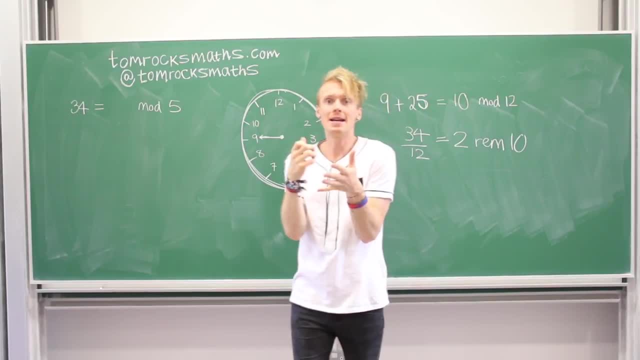 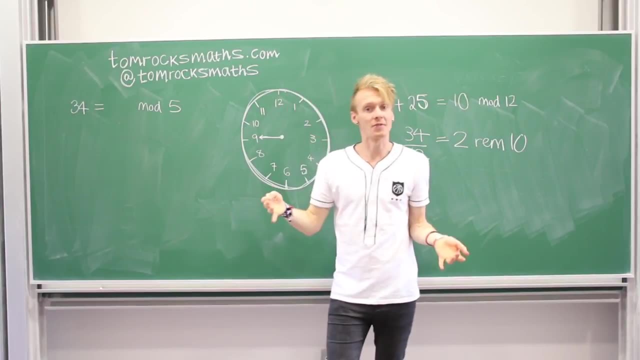 thing. so you have 34, and then you think, right, how many lots of 5s go into 34, that number? well, six fives would give you 30, and then there's four left, so the answer is going to be four. it's sort of you're just thinking about it like how. 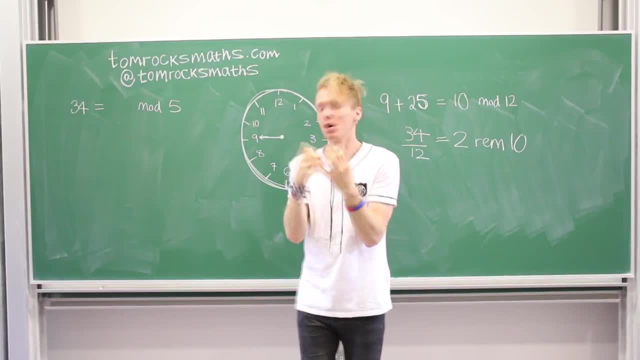 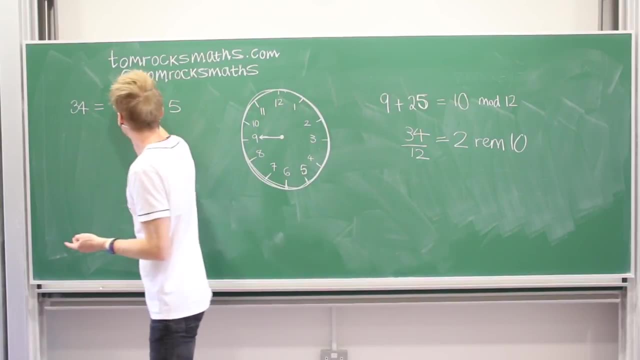 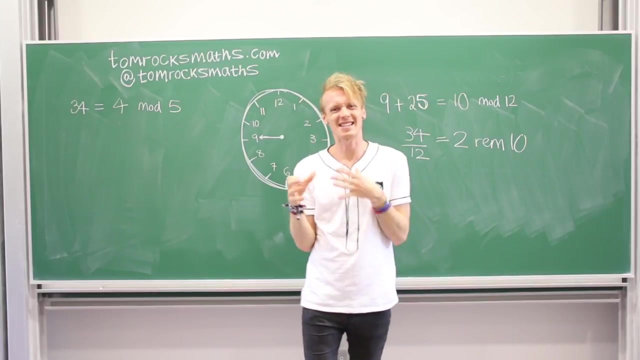 many, lots of your number, your five, your modular number go into the number you want to work out, and then what's that remainder? so in this case it's just four and it's really quite as simple as that. it sort of sounds tricky and it looks tricky, I think, modular arithmetic because it's a little bit different. 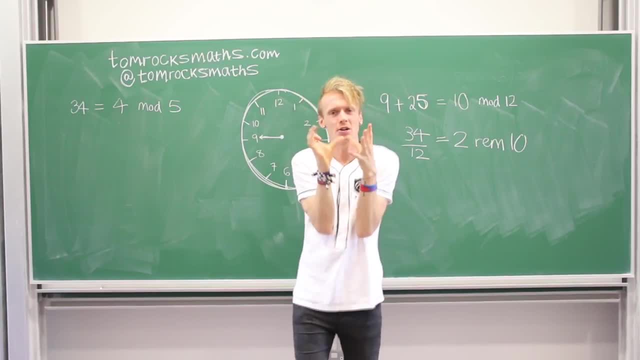 but all you're really doing is just you take your number that you want to write in a particular modular form and you just say: how many times does the modular number divide the number I'm interested in? how many times does 5 go into 34? well, 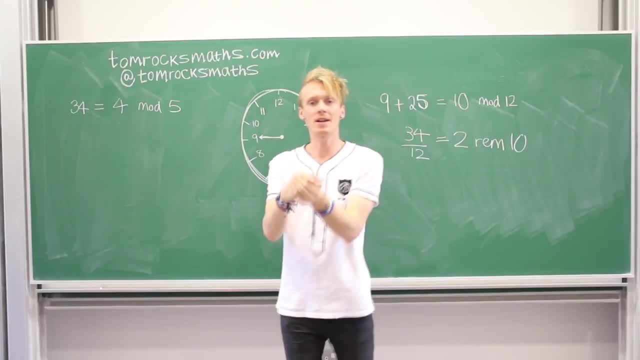 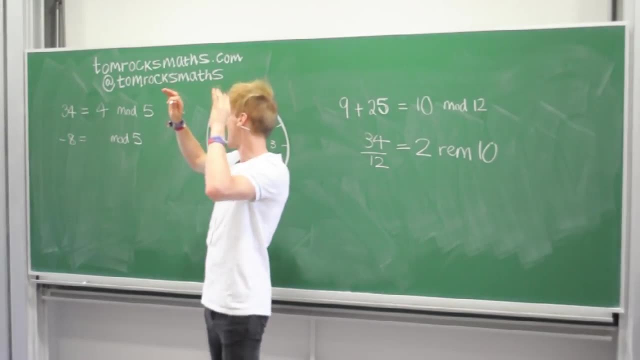 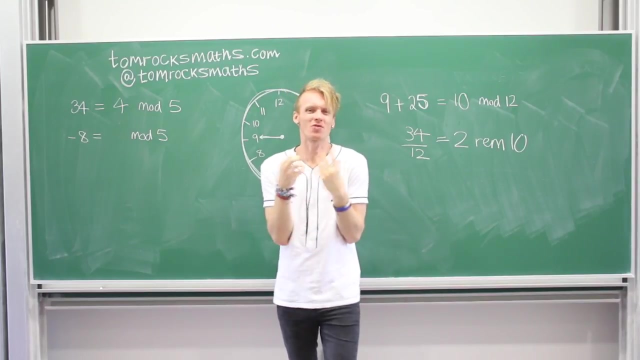 it'll go in six times to get 30 and there's four left remainder, for the answer is 4, and it works the same even with negative numbers. so let's look at minus 8. what is minus 8 mod 4- 5? there are a couple of ways you can approach, sort of trying to work this out. 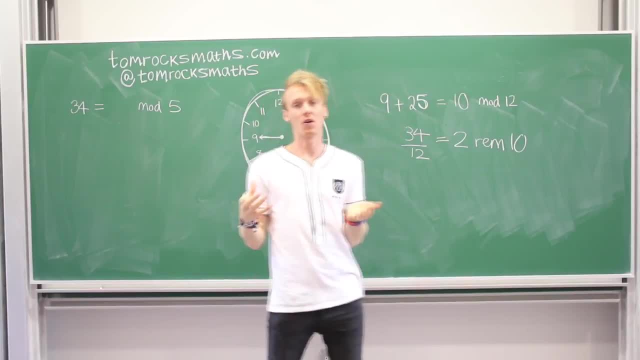 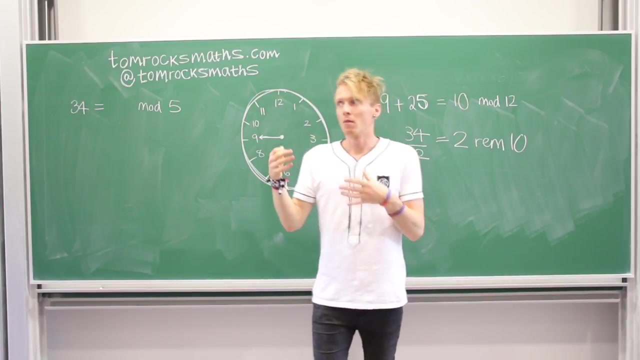 same way. so, like before, we were seeing how many 12s go into 34.. You just do exactly the same thing, so you have 34, and then you think right, how many lots of 5 go into that number? So the answer is going to be 4.. It's sort of you're just thinking about it like how many lots of your number. 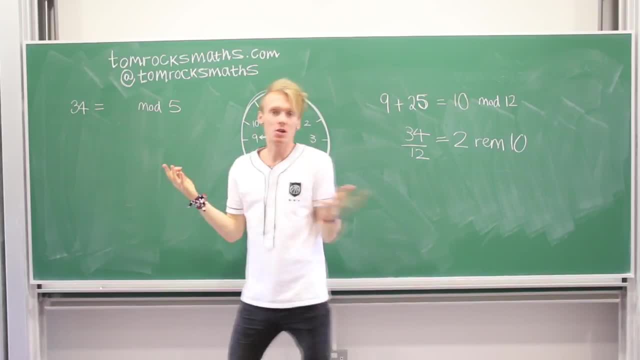 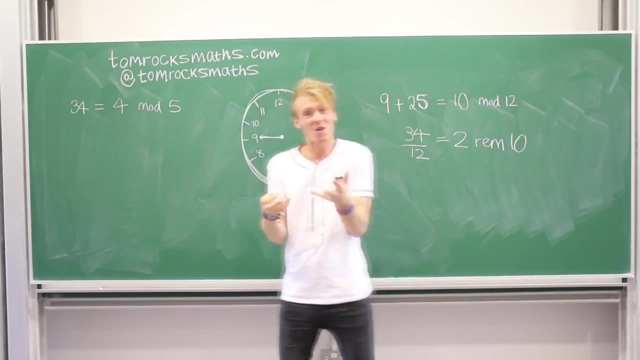 your 5, your modular number, go into the number you want to work out, and then what's that remainder? So in this case it's just 4 and it's really quite as simple as that. it. it sort of sounds tricky and it looks tricky, I think, modular arithmetic, because it's a little bit different. but all you're really 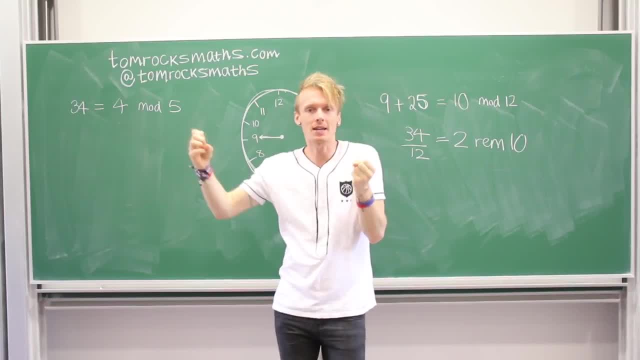 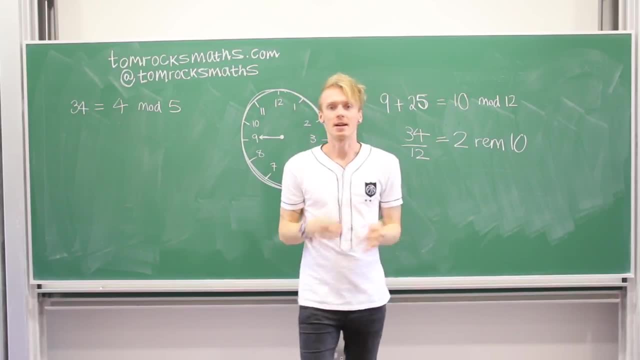 you take your number that you want to write in a particular modular form and you just say: how many times does the modular number divide the number I'm interested in? How many times does 5 go into 34?? Well, it'll go in six times to get 30. and there's four left, Remainder 4. the answer is 4 and it works. 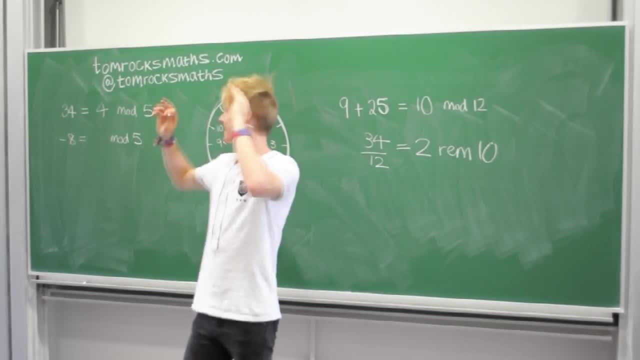 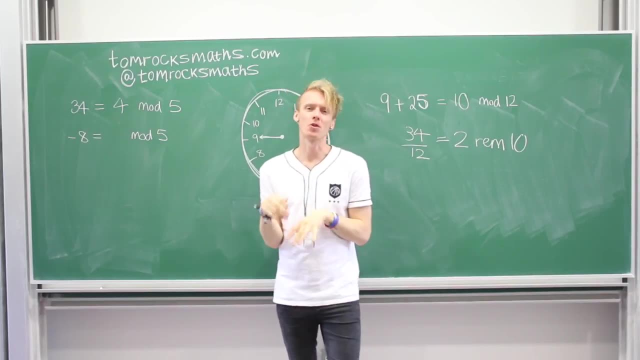 the same even with negative numbers. So let's look at minus 8.. What is minus 8 mod 5?? There are a couple of ways you can approach, sort of trying to work this out if you don't see it straight away. So 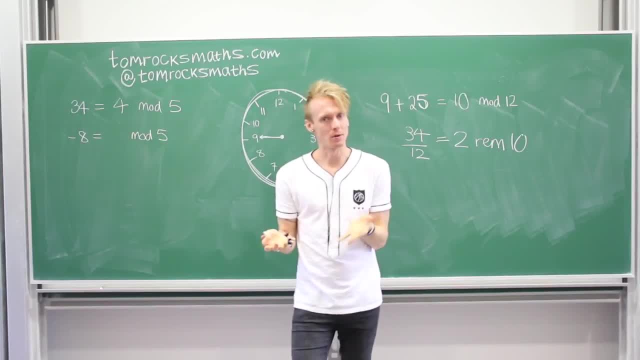 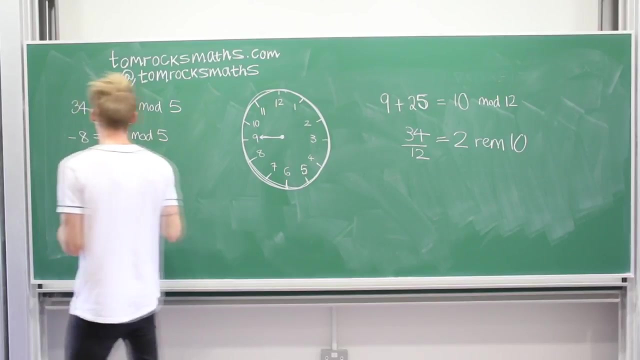 you can think right. well, positive 8, for example, one lot of 5 goes into 8 and there's a remainder of 3. So because we're here thinking minus 8, then this would also be the same as minus 3. And this is a correct statement. this is fine. this is completely true mathematically. but 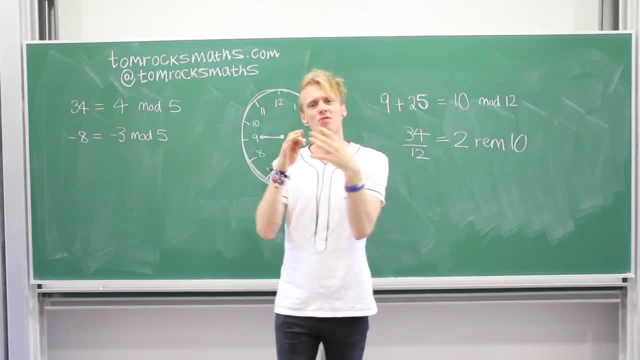 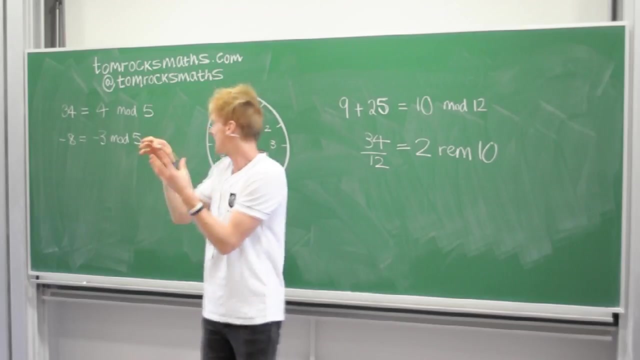 what we try to do in modular arithmetic is to write our answers in terms of the positive integers up to your modular number. So in the case of mod 5, you want your answer to be either 0,, 1,, 2,, 3 or 4.. Like your clock, you're counting 1,, 2,, 3,, 4,, 5, 6, all the way around to 12, and then you start. 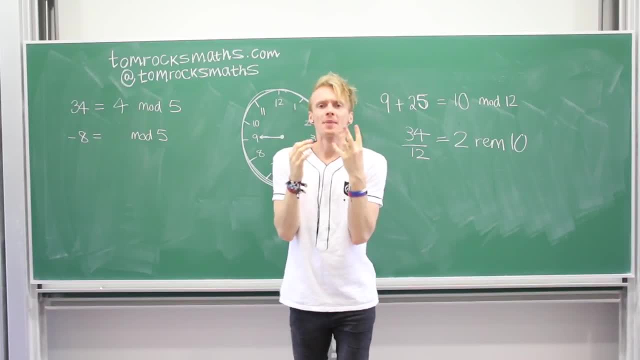 if you don't see it straight away. so you can think: right, well, positive 8. for example, one lot of 5 goes into 8 and there's a remainder of 3. so because we're here thinking minus 8, then this would also be the same as minus 3, and this is. 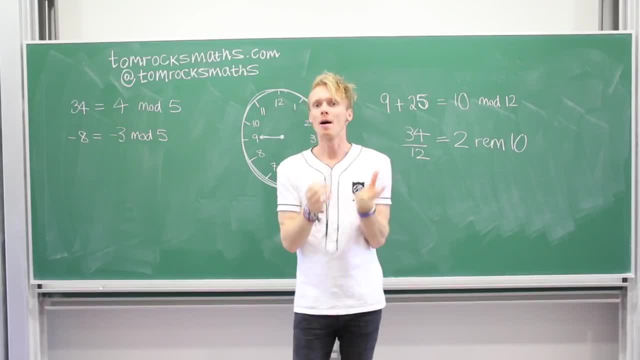 a correct statement. this is fine. this is completely true mathematically. but what we try to do in modular arithmetic is to write our answers in terms of the positive integers up to your modular number. so in the case of mod 5, you want your answer to be either 0, 1, 2, 3 or 4. 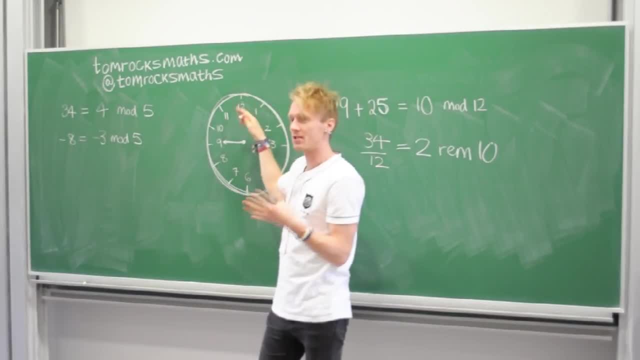 like your clock. you're counting 1, 2, 3, 4, 5, 6, all the way around to 12, and then you start again. you're doing the same here, but you're going from naught to 4 and then back to naught. 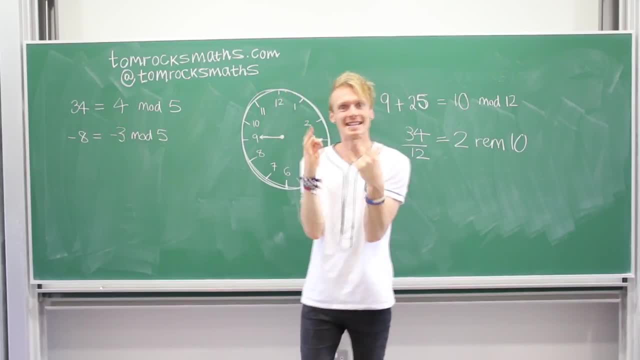 so rather than writing this as minus 3, which of course isn't inside that naught to 4 interval, we want our answer to be: what you can do is just add 5 until you get into that interval. so minus 3 plus 5 gives you 2, and that does indeed lie. 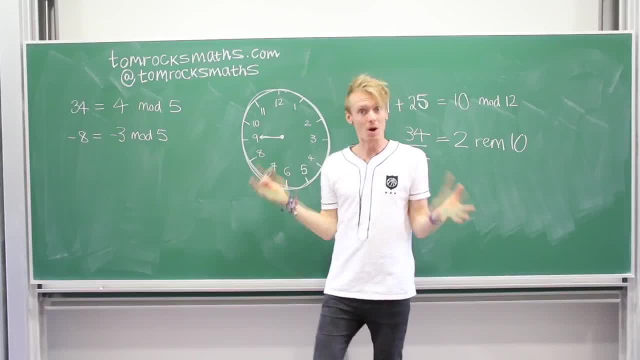 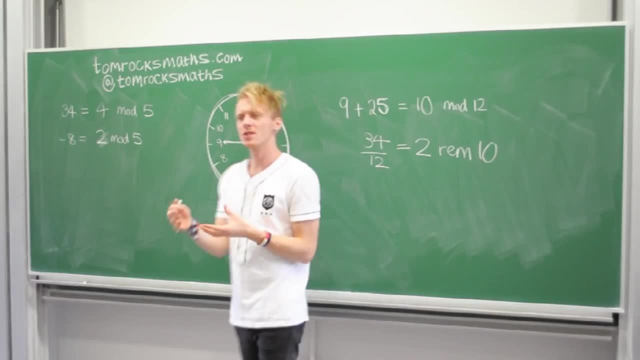 between the interval of naught to 5 that we want. so here the answer is also just 2 and it looks a bit neater. and I also gave another little trick there in working that out when you're working in modular arithmetic and that's to add the modular number over and over again to your number, or 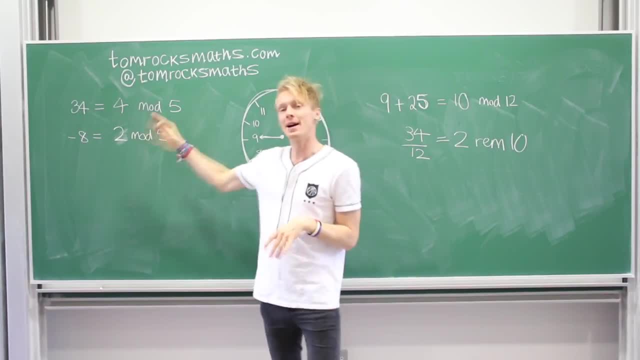 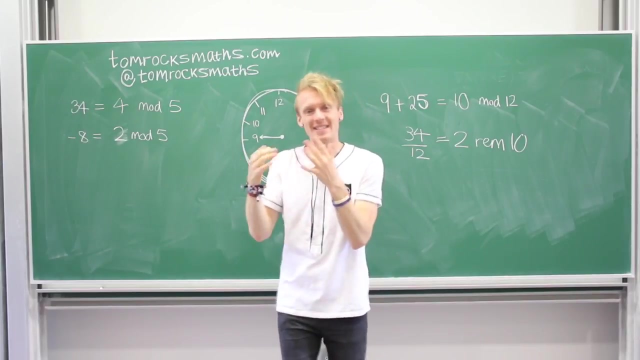 similarly you can subtract it. so with a number like minus 8, you can just add 5, because 5, remember, is 0 mod 5. so it's like if you've got the number 3 and then you add 0, you're still at 3. well, adding 5 in mod 5 is the same as the. 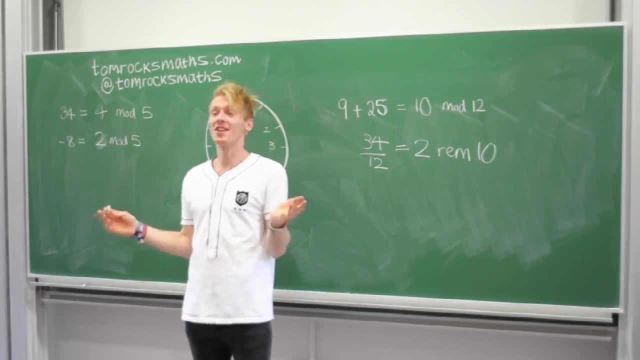 number of times you've added 0 doesn't change your answer, and that's pretty much all there is to it. it's. it's not really any harder than normal arithmetic that you've been taught at school or university. it's just you have to think a. 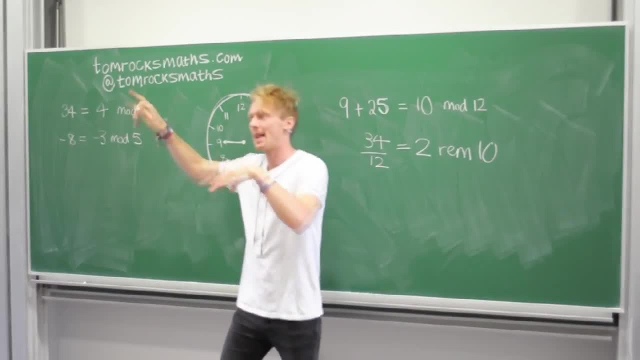 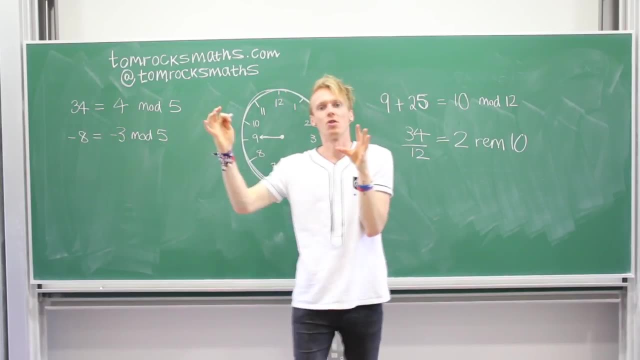 again, You're doing the same here, but you're going from 0 to 4 and then back to 0. So, rather than writing your answer to be 0 to 4, which of course isn't inside that 0 to 4 interval- we want our. 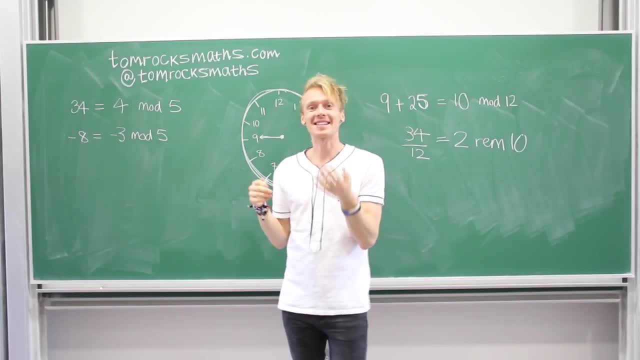 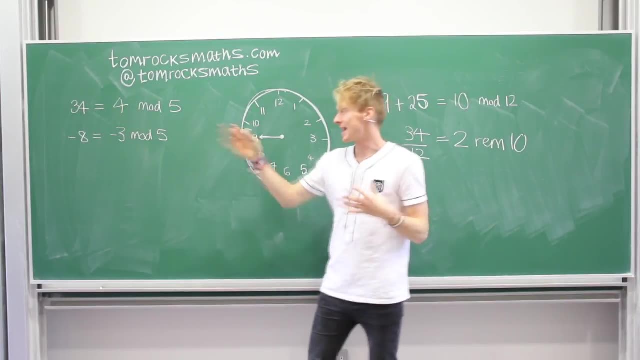 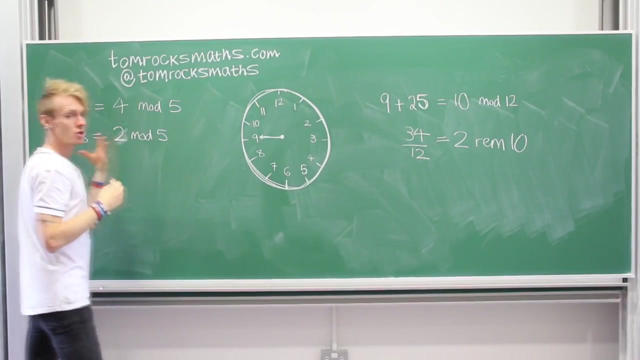 answer to be: what you can do is just add 5 until you get into that interval. So minus 3 plus 5 gives you 2, and that does indeed lie between the interval of 0 to 5 that we want. So here the answer is also just 2, and it looks a bit neater, And I also gave another little. 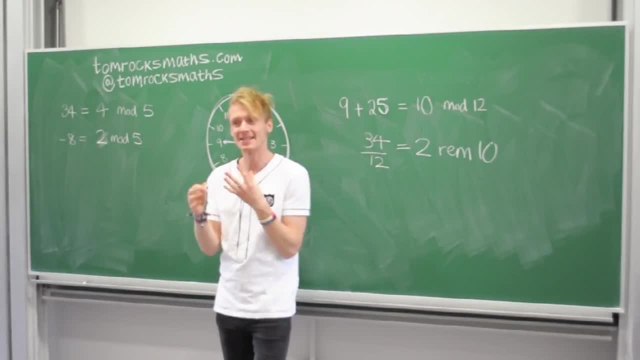 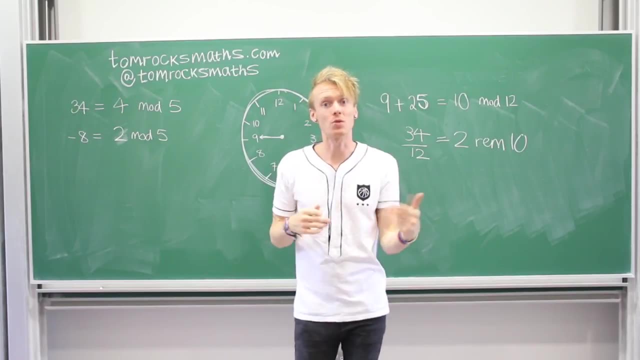 example of how you can write your answer. that's out when you're working in modular arithmetic, and that's to add the modular number over and over again to your number. or similarly, you can subtract it. So with a number like minus 8, you can just add 5, because 5, remember, is 0 mod 5.. So it's like if 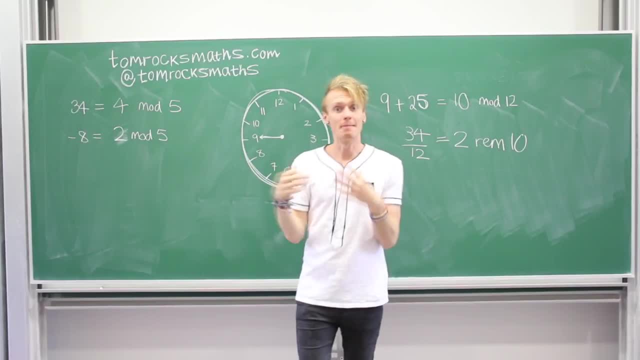 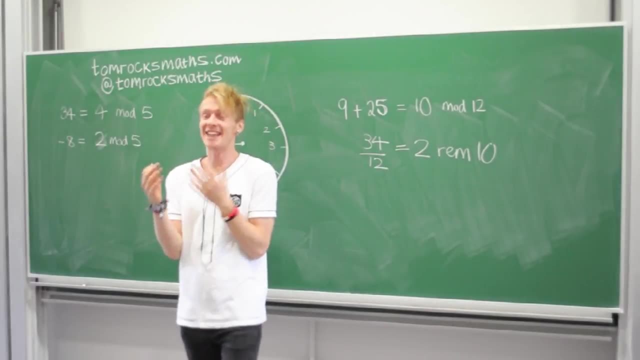 you've got the number 3 and then you add 0, you're still at 3.. Well, adding 5 in mod 5 is the same as your answer, And that's pretty much all there is to it. It's not really any harder than normal. 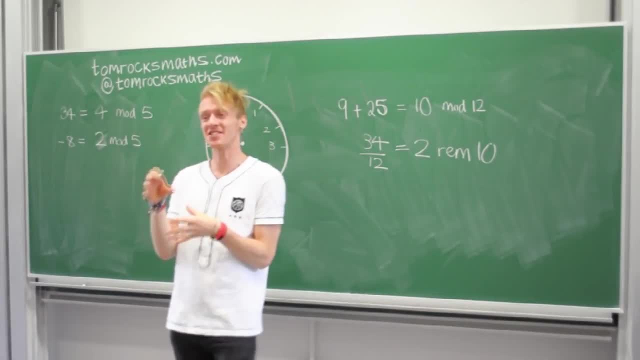 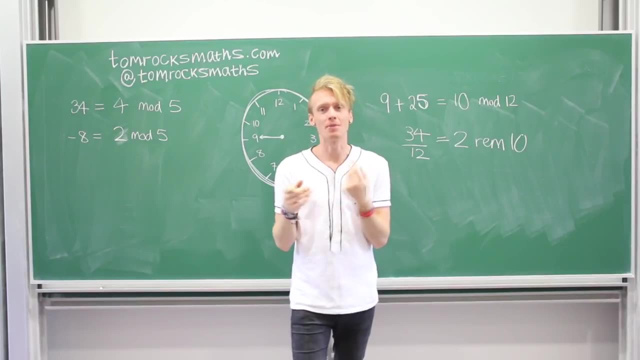 arithmetic that you've been taught at school or university. It's just you have to think a little bit more. but you're not really doing anything different. The operations of addition, subtraction, multiplication, division, they all work exactly the same way. So you do the normal operation to. 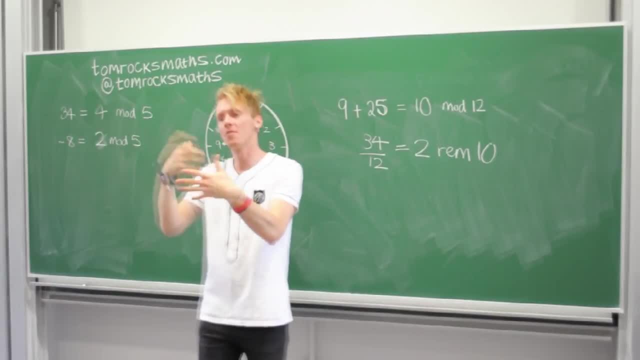 get your answer, and once you have that answer, you then just convert it into the correct form by dividing it by a number. So that's pretty much all there is to it. It's not really any harder than normal arithmetic that you've been taught at school or university. It's just you have to think a little. 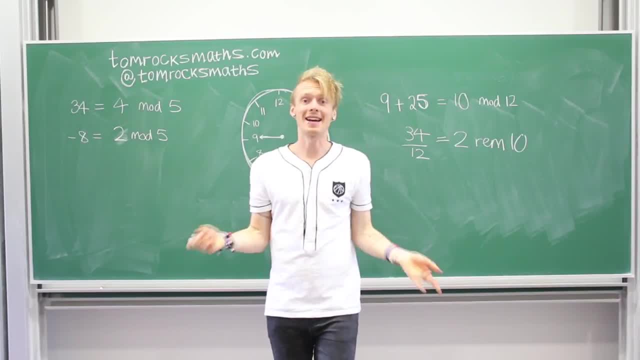 bit more, but you're not really doing anything different. So you do the normal operation to get your answer, and once you have that answer, you then just convert it into the correct form by dividing by your modular number and working out the remainder. It's really as simple as that. So let's do one. 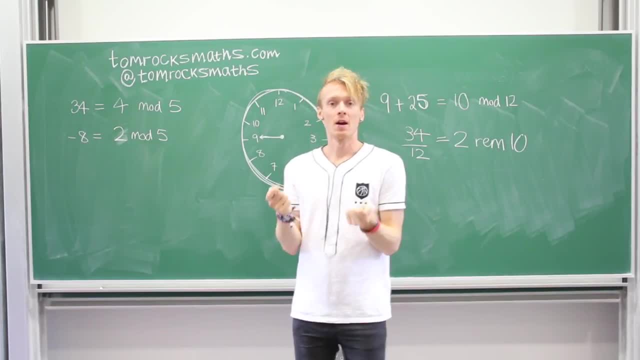 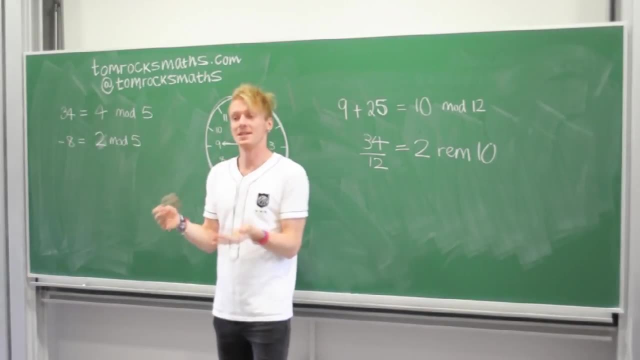 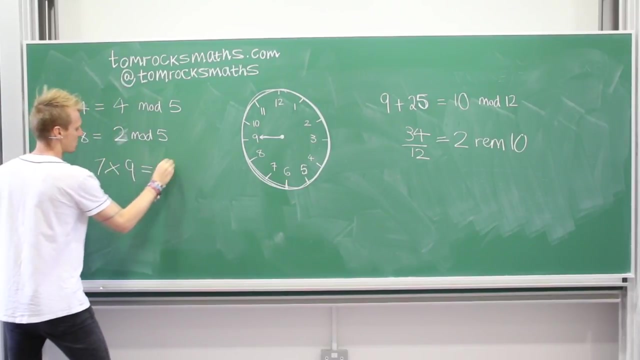 final example: Say 7 times 9 and we want to work out what is 7 times 9 mod 21.. So, to start with, you just do 7 times 9 in the normal way, So 7 9- 63. So 7 times 9 equals 63. And we want to know what. 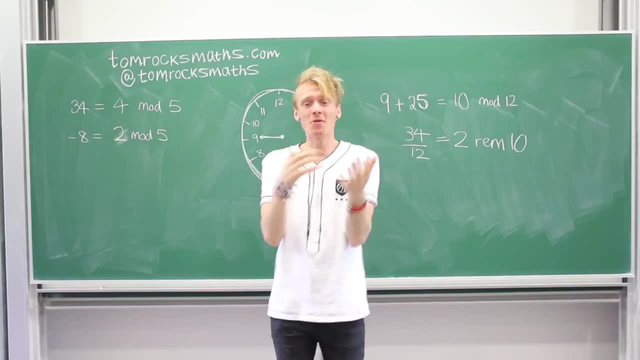 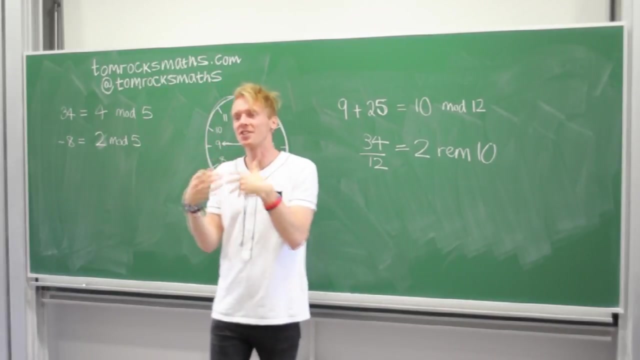 little bit more, but you're not really doing anything different. the operations of addition, subtraction, multiplication, division, they all work exactly the same way. so you do the normal operation to get your answer. once you have that answer, you then just convert it into the correct form by dividing by your modular number and working out the 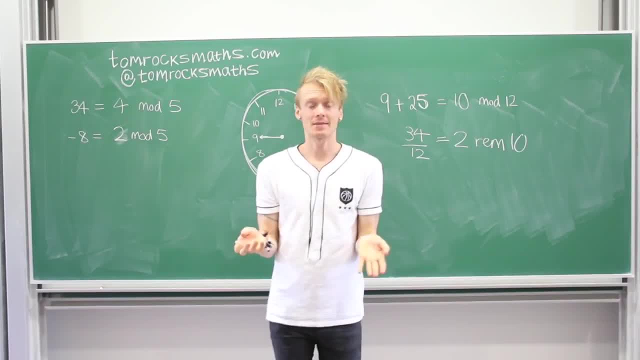 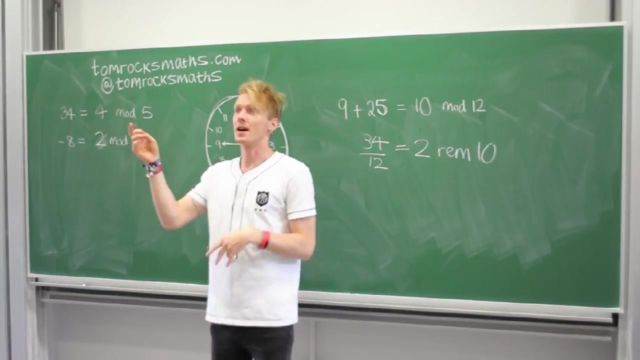 remainder it's. it's really as simple as that. so let's do one final example. say 7 times 9, and we want to work out what is 7 times 9 modular 21. so to start with you, just do 7 times 9 in the normal way. so 7, 9, 63. so 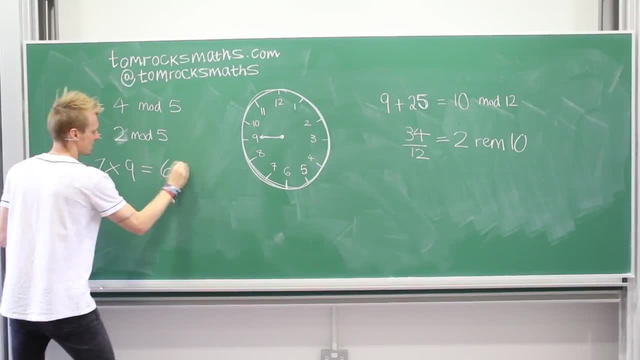 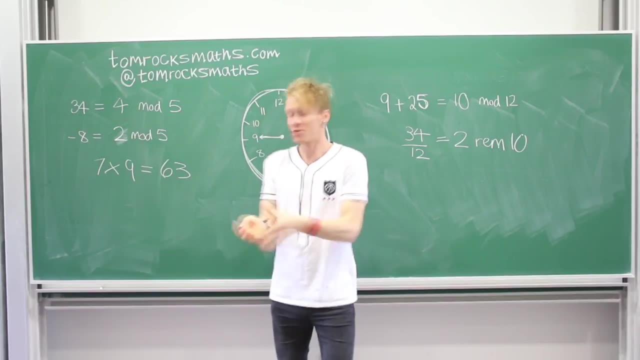 7 times 9 equals 63, and we want to know what this is. modular 21. well, you just get your answer and then you say: right, how many 21s go into 63? well, 63 is exactly 3- lots of 21. so 63 divided by 21 is exactly 3. 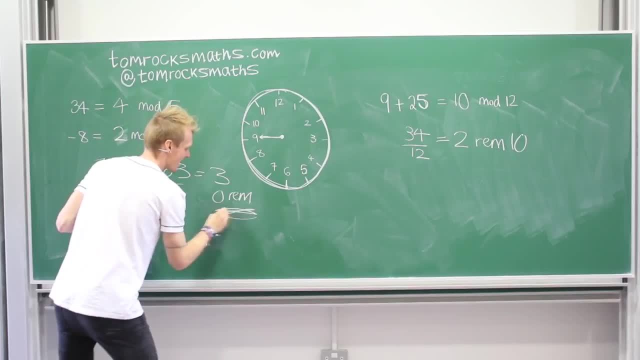 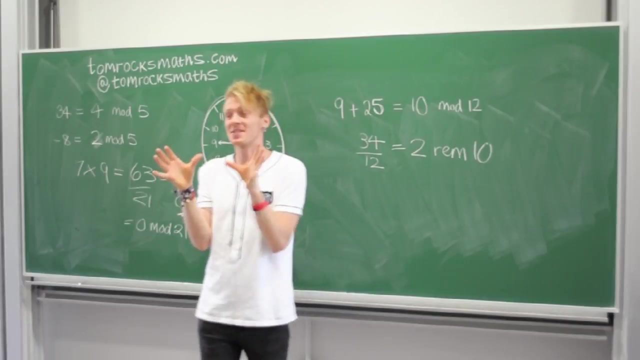 with 0 remainder. and this bit here is what's key. the fact that there's 0 remainder means that the answer here is simply 0 mod 21. so have a go yourselves. just take a simple set of sums, simple set of multiplications, and just try and convert them into modular arithmetic. just pick a. 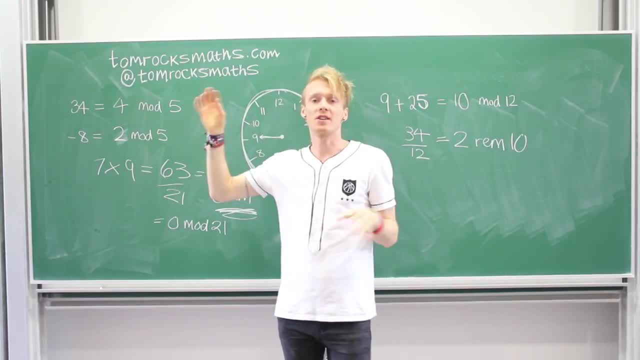 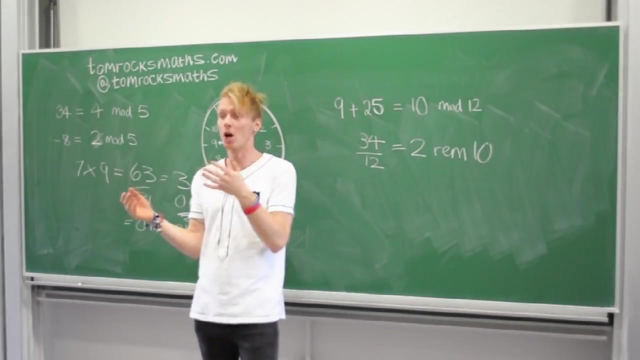 number and say: right, I'm going to work out these 10 sums in, say modular 63, and the more practice you do, the more it will become second nature and the more you'll realize that module arithmetic is not really that much harder than normal arithmetic. so thank you everybody for watching. I hope I've answered the. 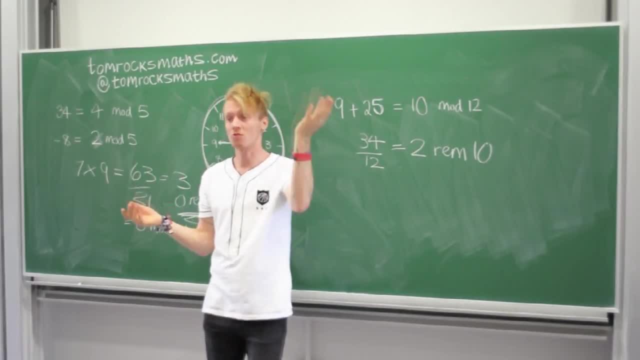 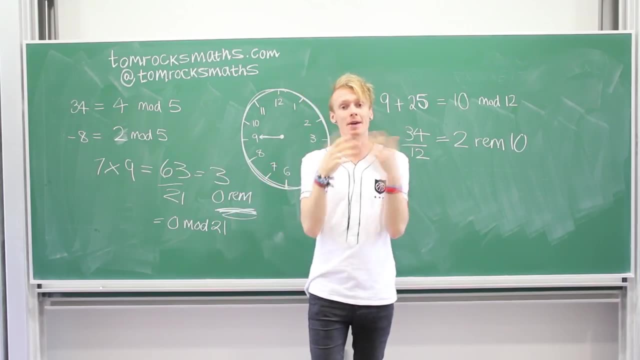 question. if you've enjoyed this video, please give me a thumbs up if you've. if you like what i'm doing, please do subscribe. that way, you'll be the first to hear when a new video becomes available, and also be sure to check out all my material on my website. 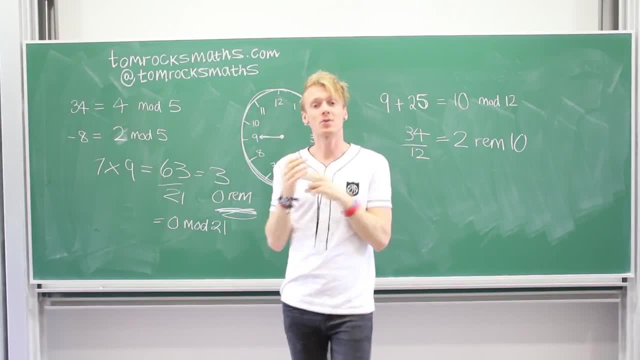 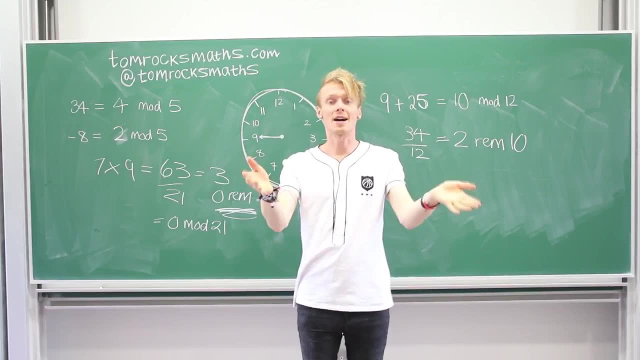 tomrocksmathscom, and also you can follow me on facebook, twitter, instagram at tomrocksmaths, and i will see you next time with another answer to a question that you guys have voted for.